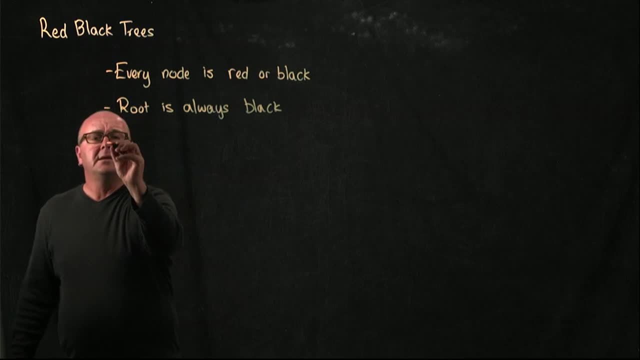 it to be black. Next to follow: New insertions are always red. We always start with things that insertions are red. If we insert something as the root node, we insert it as red, but we immediately make it black. Next. 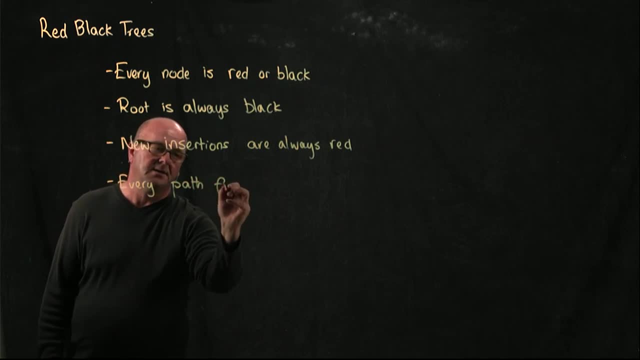 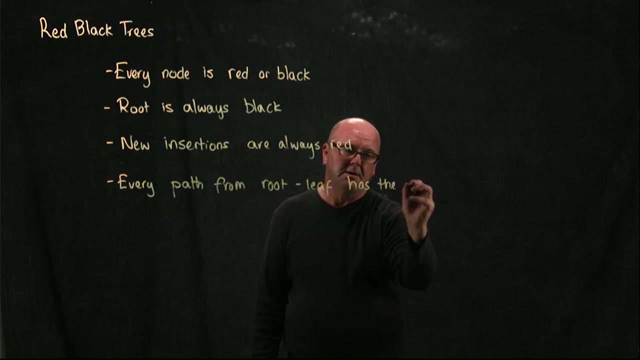 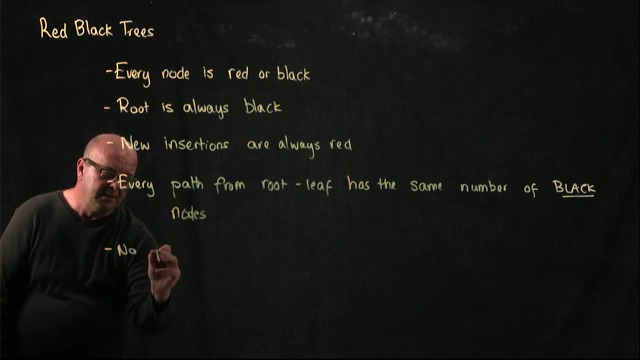 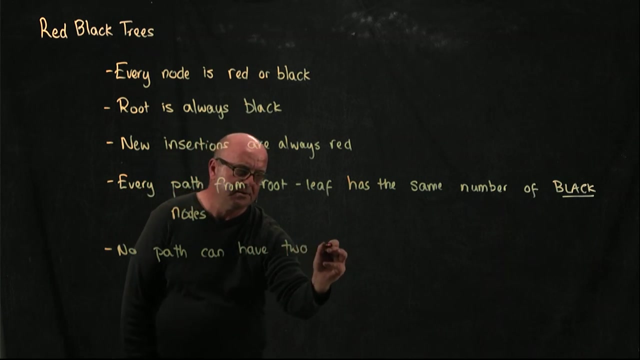 every next path, from root to leaf. So every possible path that we can take through our tree has the same number of black nodes. No path can have two consecutive red nodes And, finally, any null node is considered to be black. So two things to notice here. 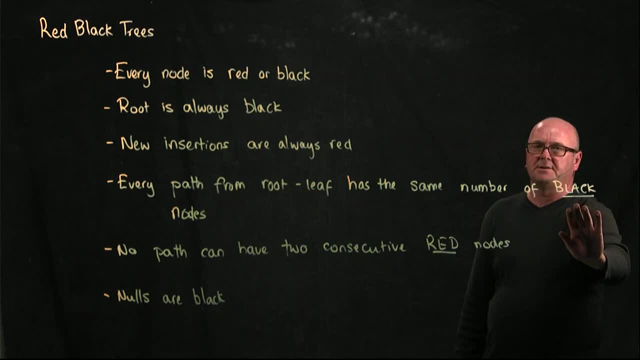 Every path from root to leaf has the same number of black nodes. That means that different paths from root to leaf can have different numbers of red nodes. That's okay. It's specifically black nodes And no path can have two consecutive red nodes. 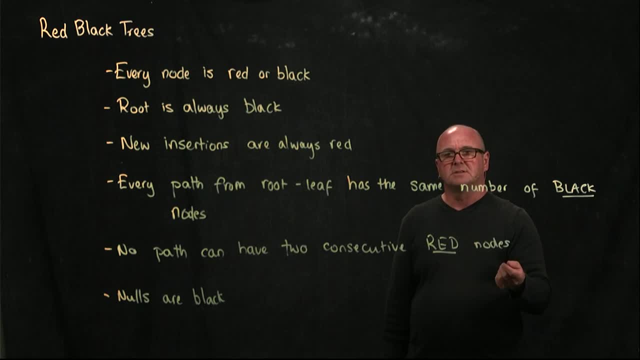 But a path can have two consecutive black nodes. That's also okay. So these are our six rules. Remember them. If I set you an exam question about red-black trees, which is quite likely, I often ask you a question which is: 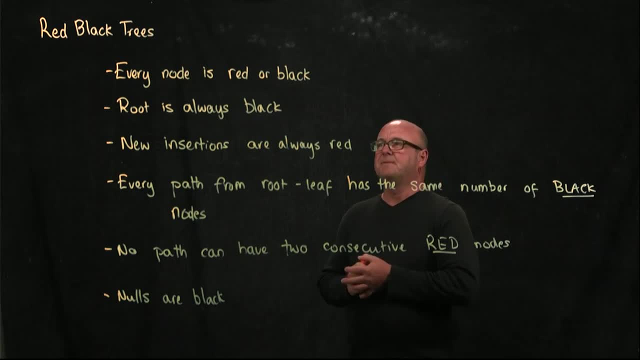 what are the six rules? People often forget every node is red or black, or that nulls are black. But these are the six rules for red-black trees. Every time we add to our red-black trees, we come back to these rules. we take a look at them. 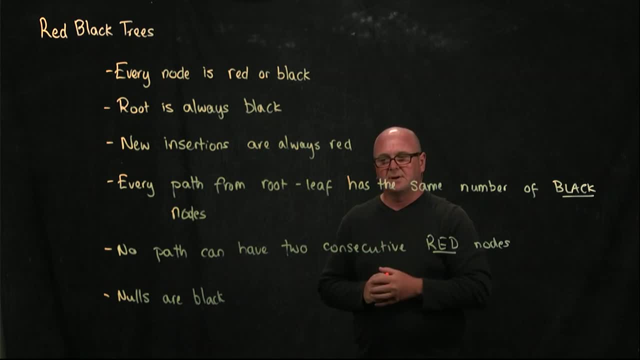 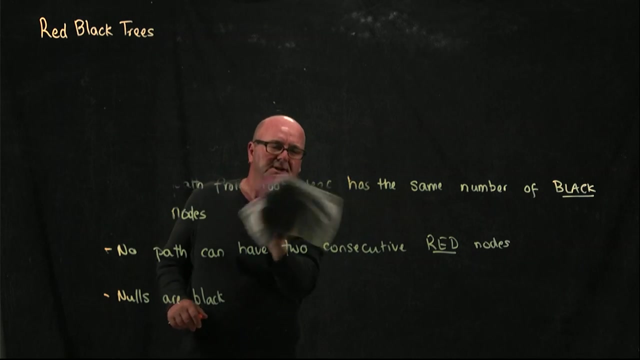 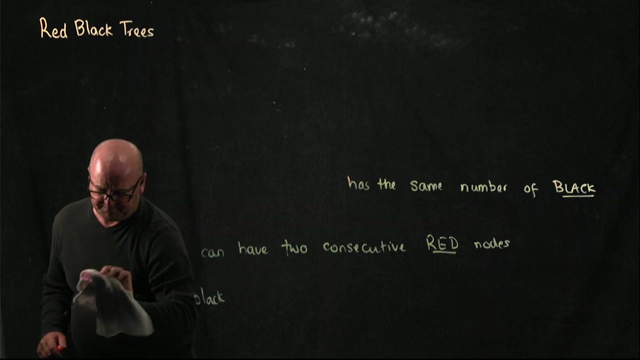 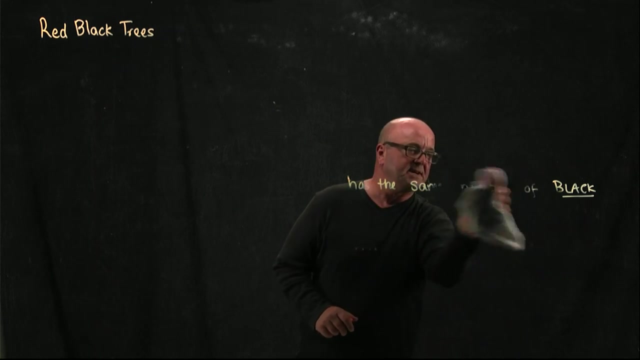 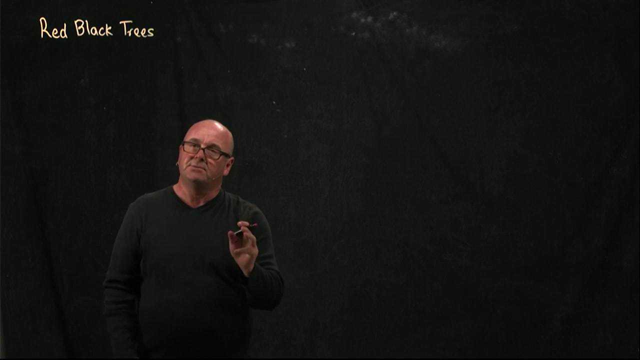 and we ask: do our trees violate these rules? What happens if our tree violates these rules? Well, we have to fix the tree. Let's take a look at how we do that fix. There's two more rules for fixing the tree. 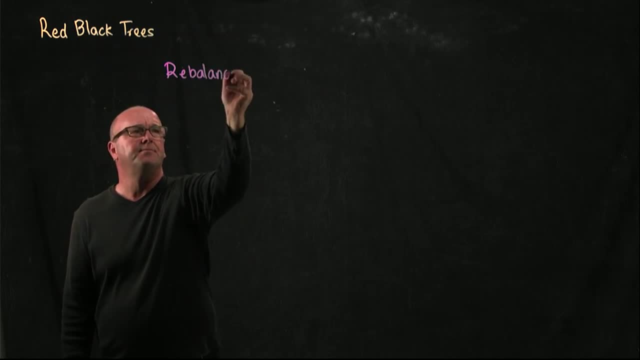 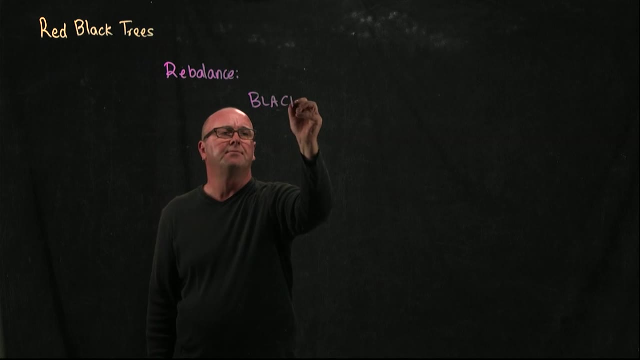 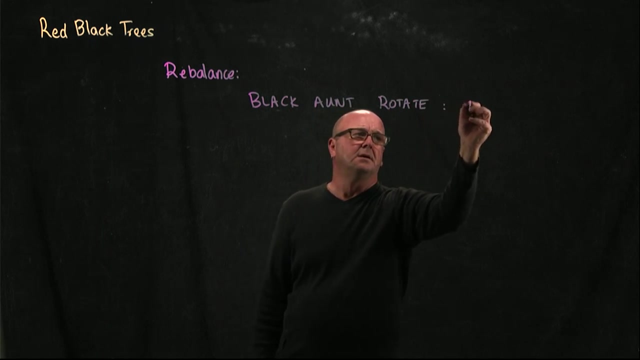 So we need to rebalance based on whether, if we have a black, aren't we rotate Black, aren't we rotate. If we have a red, aren't we color flip? So I don't have black and red, so I'm going to use alternate colors. 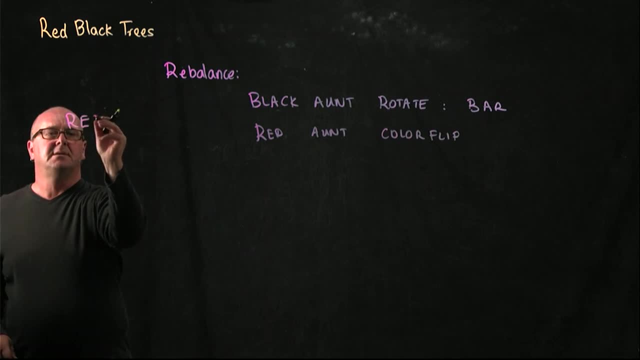 I'm going to use red for red and I'm going to use blue for black. Okay, So after we do either a rotation or a color flip, after that we then need to resolve the colors on the tree, And you'll see what I mean by this. 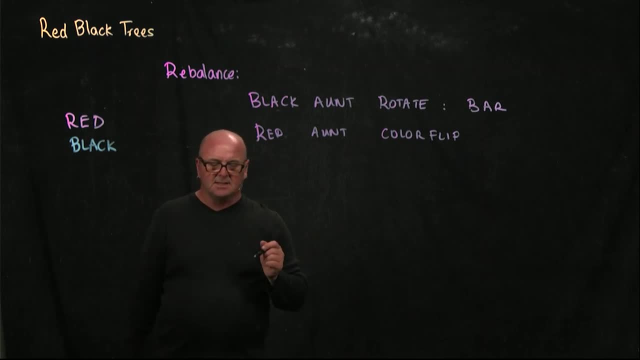 when I go through an example. But the rule is that after a rotation, the three nodes that we're working on end up as black, red, red. Okay, So the parent is black and the two children are red. In contrast,